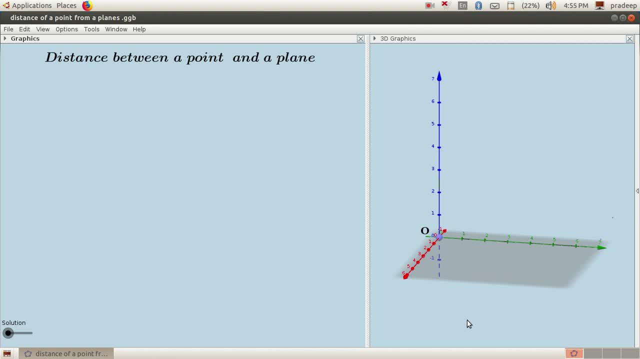 Hi students, the concept we are going to discuss here is about the distance of a point from a plane. Here we have a point P with the position vector vector A and a plane pi 1, whose vector equation is given by vector r, dot, n, cap is equal to d, where d is the distance of this plane from origin. 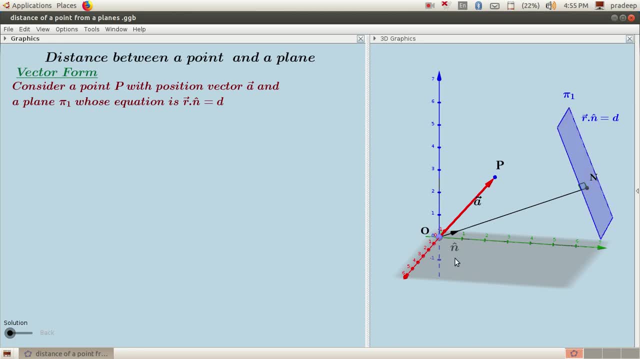 and n cap is the unit normal vector. We have to find out the distance of this point from this plane. for that we consider another plane which is parallel to the first plane and is passing through the point P, Since these two are parallel to each other. the unit normal vector, n cap, is the 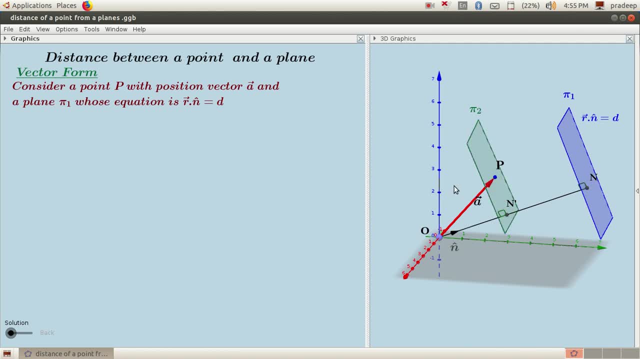 unit normal vector of the second plane also. So this equation can be written just like this: vector r dot n cap is equal to d R minus vector A dot n cap is equal to 0.. That is, vector r dot n cap minus vector A dot n cap is equal to 0. 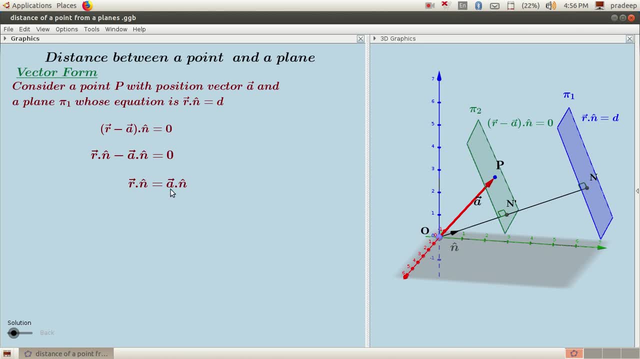 That is, vector r dot n cap is equal to vector A dot n cap. Here, this is of the form. vector r dot n cap is equal to d, Just like this, where d is the distance from origin. Therefore, the distance of the second plane from origin is obtained by: 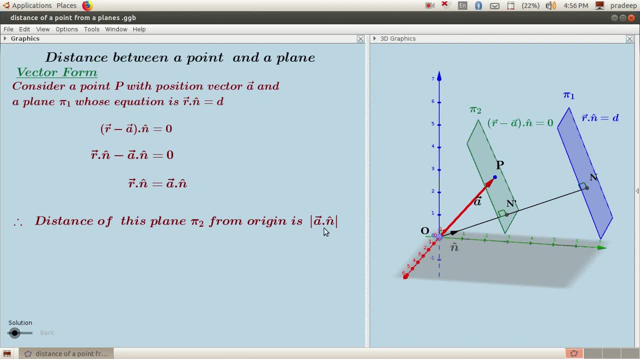 the modulus of this, That is equal to modulus of vector a dot n, cap. This is the distance of the second plane from origin. This is the distance of the first plane from origin. Therefore, in order to find out the distance between these planes, 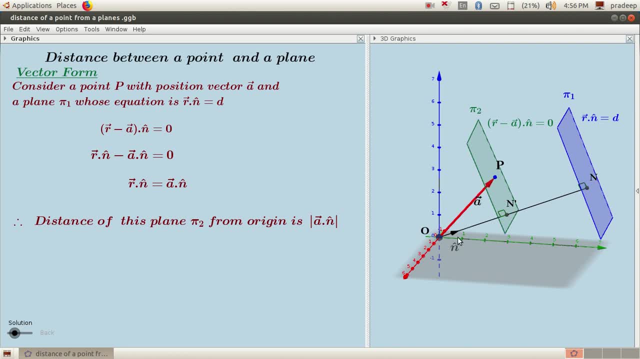 is the difference between these two. That is, first, distance is d. second, distance is modulus of a dot n cap. Therefore, the distance between these planes, n dash, n, that is o n minus o n dash, that is equal to p, q. So, in order to find out the distance between this point and this plane, 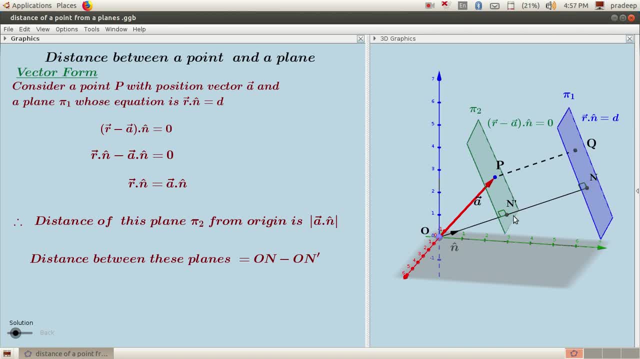 it is enough to find out o n minus o n dash. That is equal to: o n is d and o n dash is equal to vector a, dot n cap. Therefore, this is the equation Here, instead of giving this equation of the plane, just like this, r, dot and cap is equal. 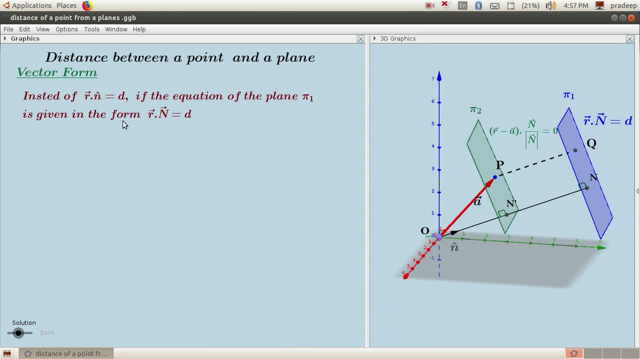 d as before, if the equation of the plane pi 1 is given in the form r dot, vector n is equal d, where vector n is the normal vector. Now this d is not the distance of that plane from origin. In order to make its distance, we have to divide throughout by the magnitude. 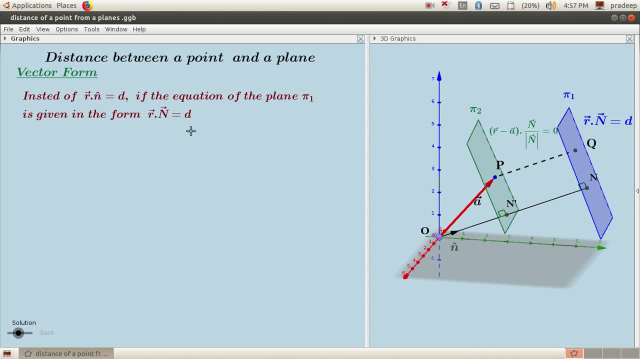 of this vector, That is, the distance of the plane from origin, is obtained by modulus of d divided by magnitude of the normal vector. This is the distance of the first plane from origin. Then, using the same concept here, this is the n cap that is obtained by dividing: 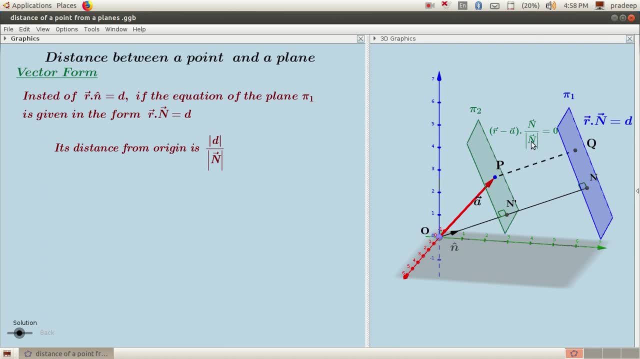 by the magnitude of this n. Therefore, the distance of this plane from origin is a dot n cap n cap is vector n divided by magnitude of vector n. This is the distance of the first plane from origin and this is the distance of the second. 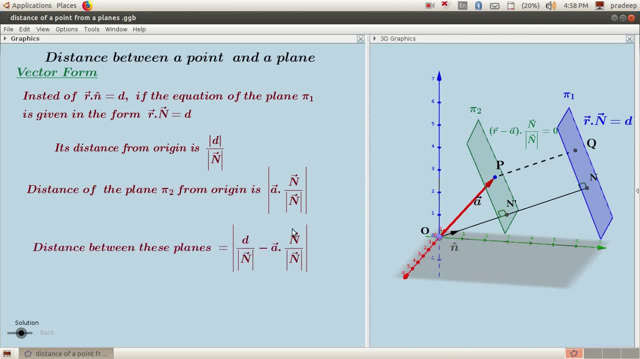 plane from origin. Therefore, distance between the planes is obtained by taking the magnitude or modulus of the difference between these, That is modulus of d divided by magnitude of vector n minus a vector dot n cap. That is n divided by magnitude of n. Here the 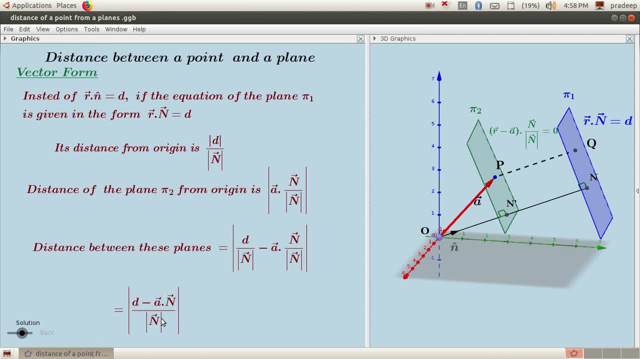 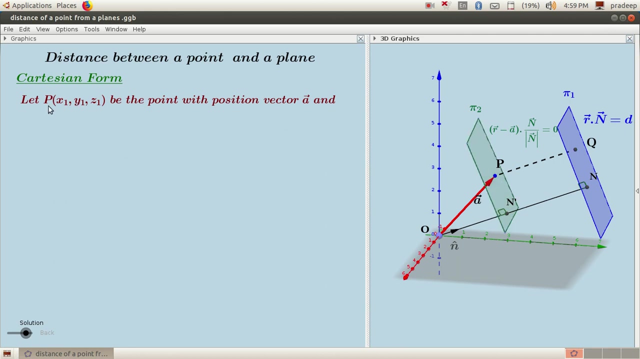 denominators are. Therefore we can write this just like this: d minus vector a, dot n divided by magnitude of vector n. and it can be written like this also Here we can move on to the Cartesian form: If the point P is a point with coordinates x1, y1, z1 and the position vector a vector. 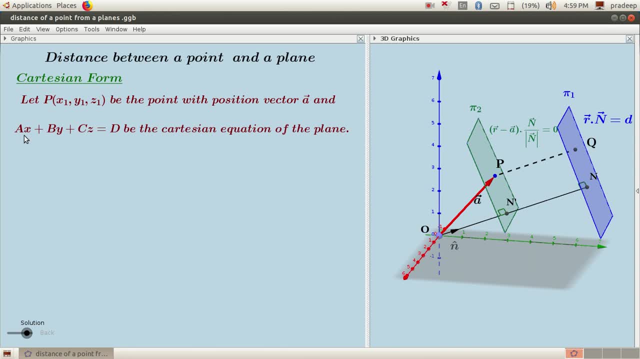 a And the equation of the plane is given by. just like this. It is in the Cartesian form: ax plus by plus cz is equal to d. Now from these coordinates we can find a is equal to xi plus yj plus zk, And from this equation we can find n is equal to ai plus bj plus.